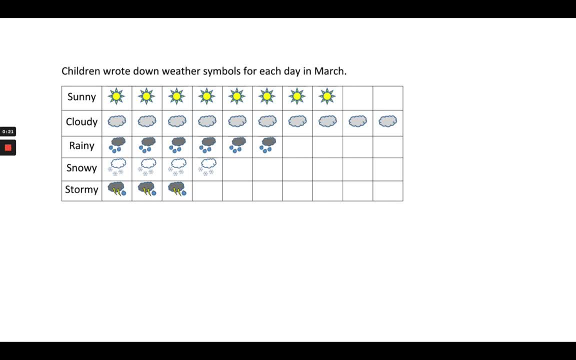 children wrote down weather symbols for each day in March. So I see my first row here is sunny and it has 1,, 2,, 3,, 4,, 5,, 6,, 7, 8 suns. So I know that it was sunny eight days in March. Okay, so for my. 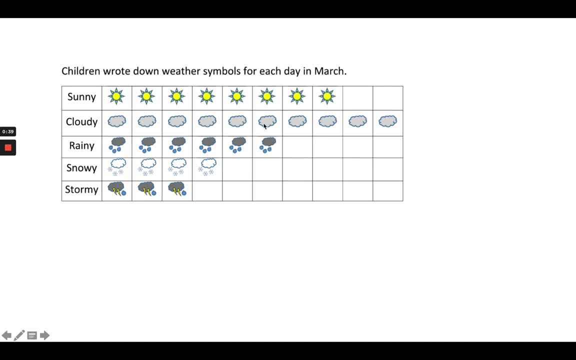 next row, I have cloudy at 1,, 2,, 3,, 4,, 5,, 6,, 7,, 8,, 9, 10 clouds. That represents 10 cloudy days in the month of March. Okay, and I have six rainy days and four snowy days and then three. 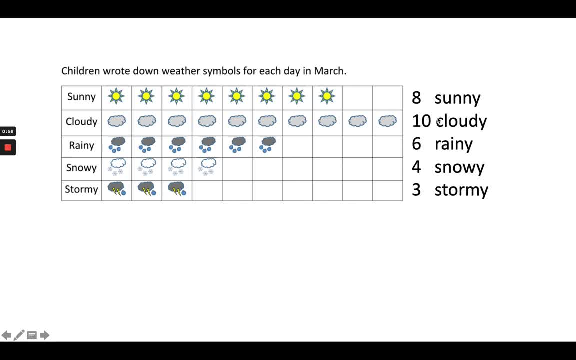 stormy days. So I know that it was sunny eight days in March. Okay. so for my next row, I have stormy days in the month of March, Okay. so each one of these symbols represents the day. So I had eight sunny days, ten cloudy days, six rainy, four snowy and three stormy. So now that I have looked, 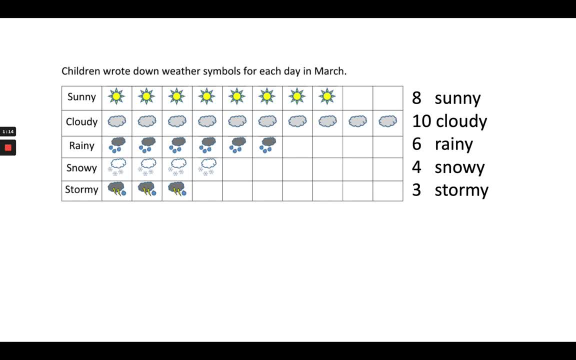 and analyzed this chart. I'm ready to answer some questions about this chart. How many days were rainy and snowy? So I need to go back and look at my chart where it says rainy and I see that there were six rainy days and three stormy. So I'm going to go back and look at my chart where it says: 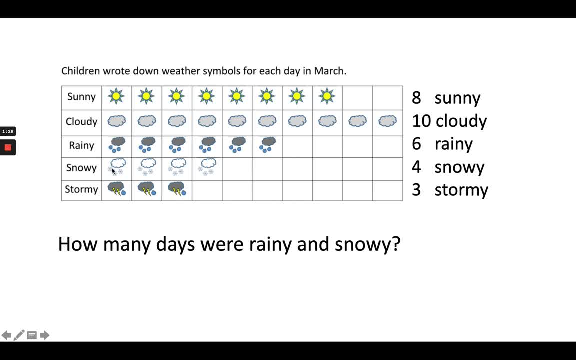 six days, and then I need to go back and find where it said snowy. There were four days that were snowy. So I know, in order to figure out how many days were rainy and snowy, I need to add six and four together to get ten. So there were ten days that were rainy and snowy in the month of. 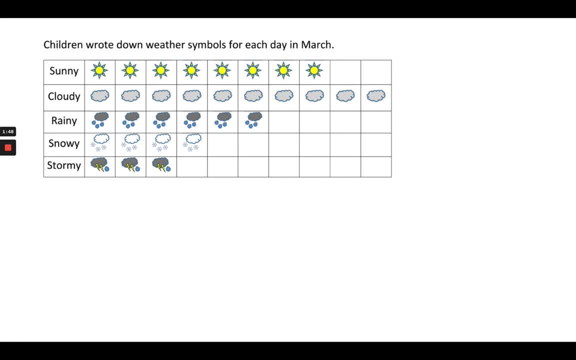 March. Okay, so let's go ahead and look at another question that can be answered with this same chart. Okay, again, we've already looked at this chart. We know the number of days that were rainy and snowy. We know the number of days that were sunny, cloudy and so forth. So how many more days were cloudy? 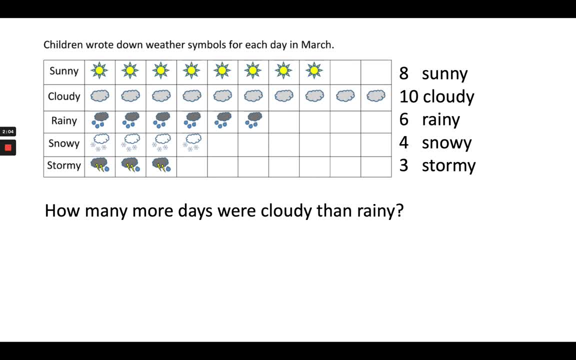 than rainy. Okay, so this time I'm not just going to be adding the number of cloudy days and the number of rainy days, because I want to figure out how many more days were cloudy than rainy. So if you look up here, I have the ten cloudy days and I have the six rainy days. but I want 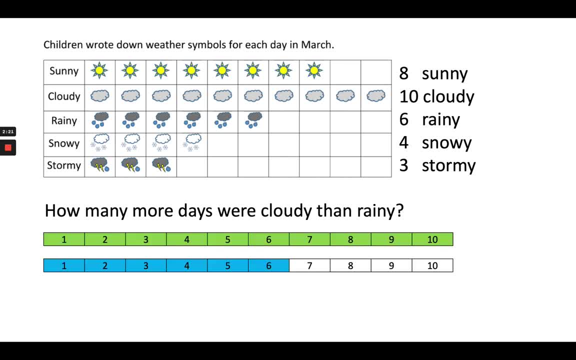 to know how many more were cloudy. Okay, so I can think about these two pieces of data Like I do a number, path and it's sort of. it's sort of shown up here. Okay, so, if I can look at this green number, path here represents the number of cloudy days and my blue one represents the 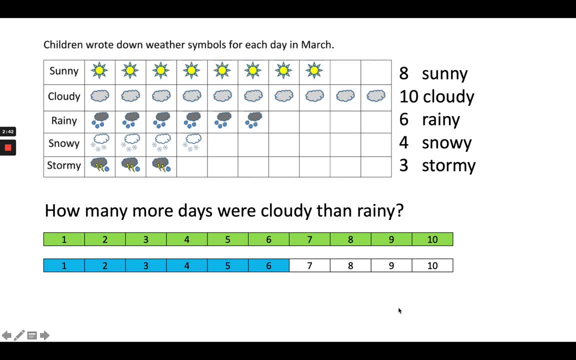 number of rainy days. So I can count one, two, three, four. So there are actually four more days that were cloudy than rainy, and I could even do that up here with my chart. I have one, two, three, four more clouds than rain, So you could also say ten minus six. So ten is the number of days that were. 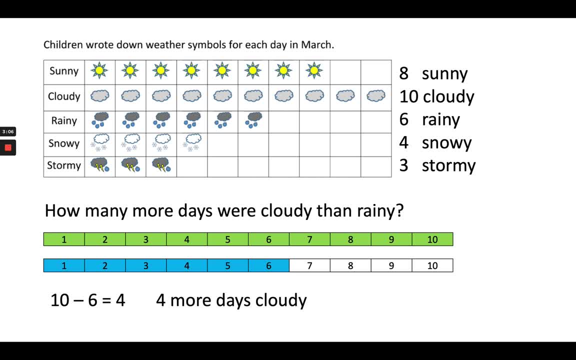 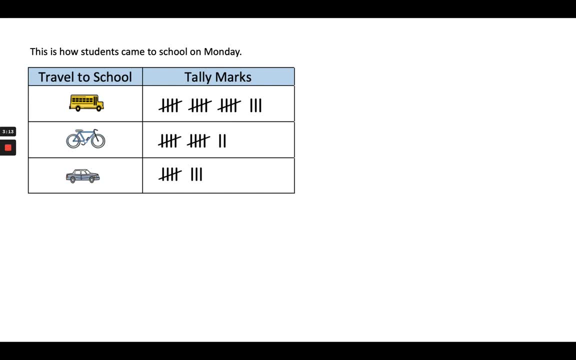 cloudy, and six was the number of days that were rainy, which would give you four, Four more days that were cloudy. Okay, all right. so let's look at a whole nother chart, and this time the chart doesn't necessarily have pictures that give me the number. It has tally marks, So let's take a look. 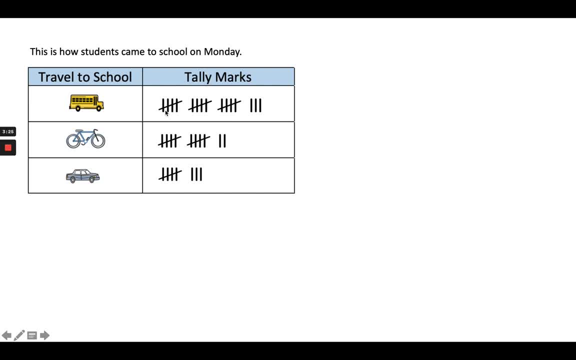 at this first little group right here. The tally mark has one, two, three, four and the fifth one is crossed over, So I know I can count by five when I use my tally marks. So this chart talks about how students came to school on Monday. 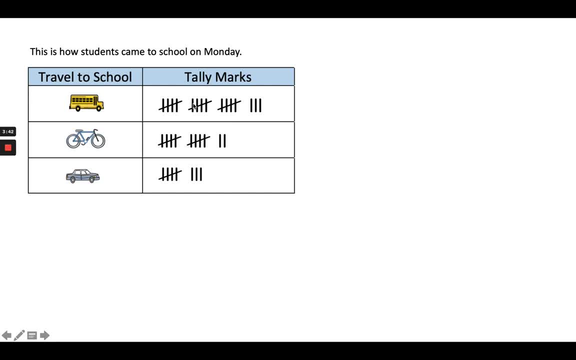 So here is a bus and I look beside it and I see five, ten, fifteen, sixteen, seventeen, eighteen. I know that 18 students traveled on the bus. So if I go down here to bike, I have five, ten, eleven, twelve. So I know I have 12 students that came on a bike And then the last one. I have a car, So I have. 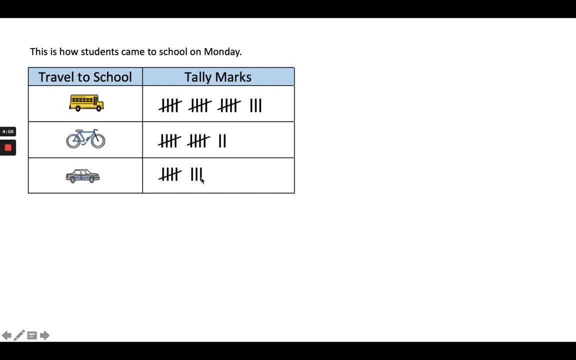 five, six, seven, eight, So eight students came by car. Okay, and so, as I've looked at that data, I've counted those tally marks. I even wrote down the numbers here beside me to help me. So now I'm ready to begin answering some questions about this chart. Okay, so how many students came in bike?